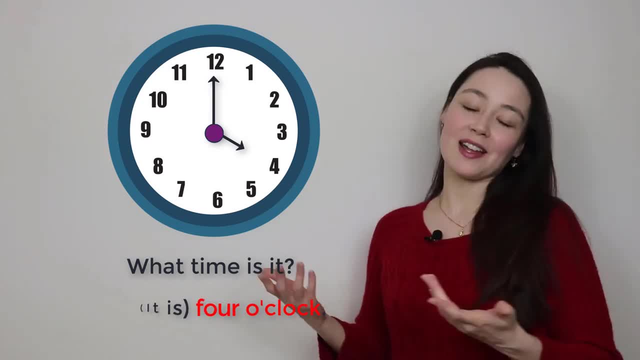 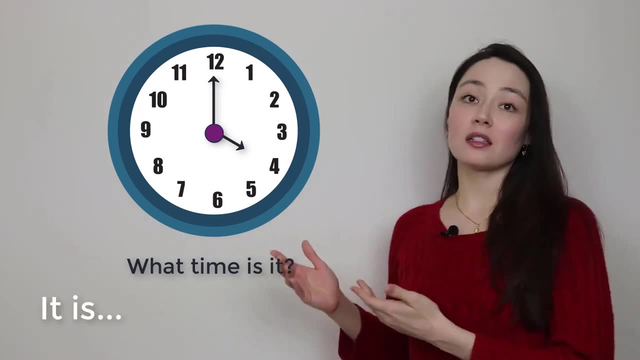 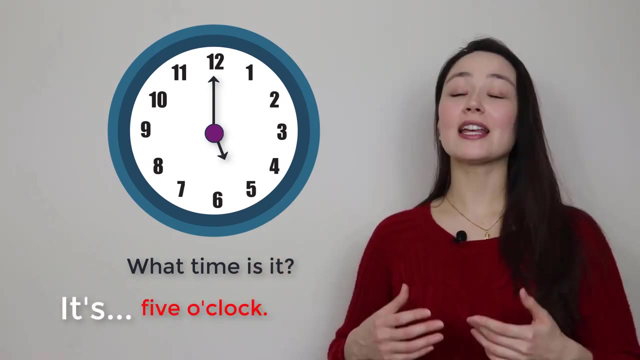 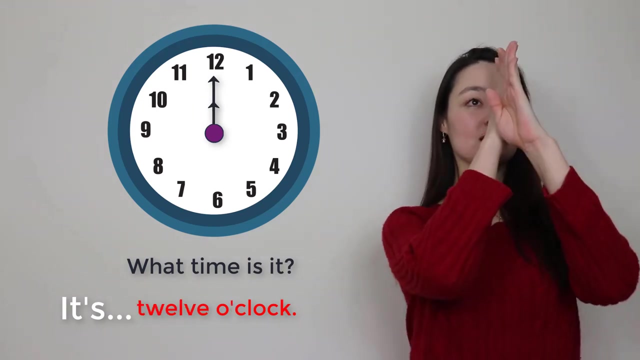 It's four o'clock. You get the idea In English, when we speak about the time, we always say it is Contracted, It's, It's o'clock. It's six o'clock, It's seven o'clock, It's twelve o'clock, If you need. 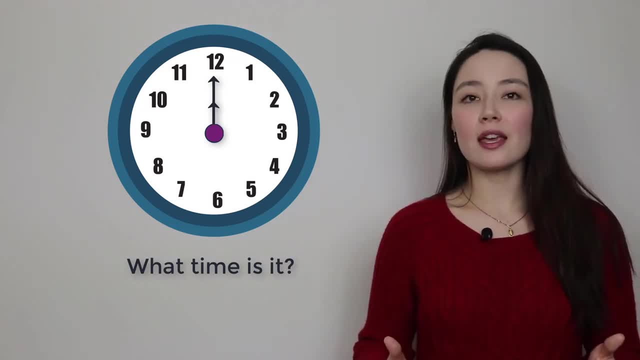 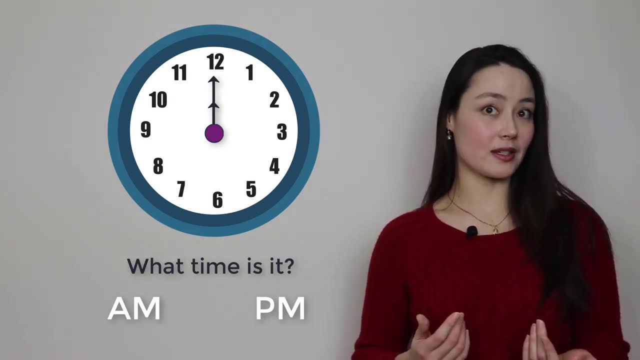 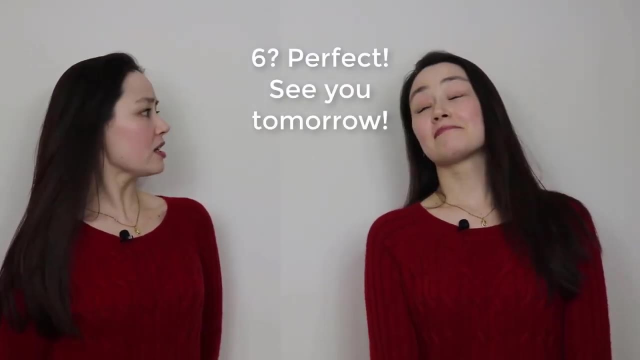 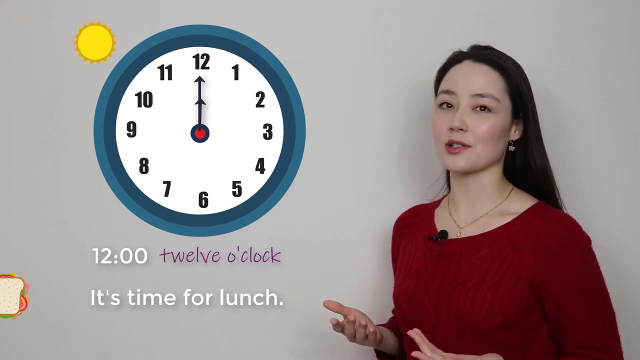 to be very specific, we can say am and pm, But normally when you're speaking it's obvious. Okay, Arnel, I need you here tomorrow at six Six, perfect, See you tomorrow. Six am am Twelve o'clock. It's time for lunch, Maybe not in your. 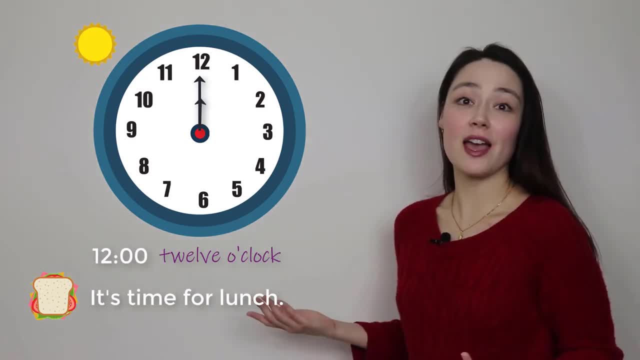 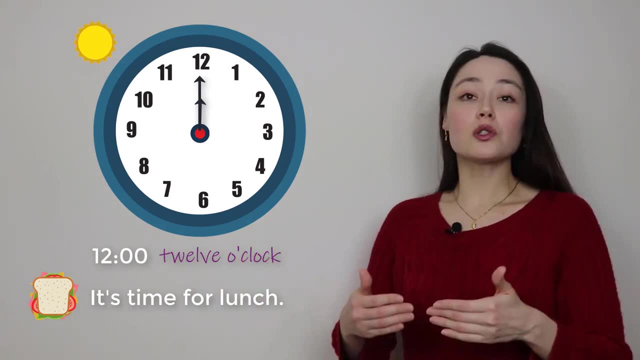 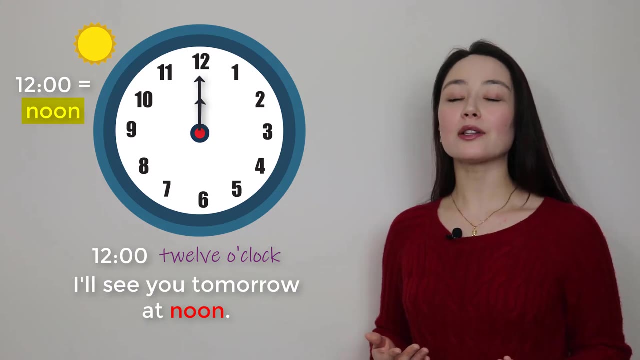 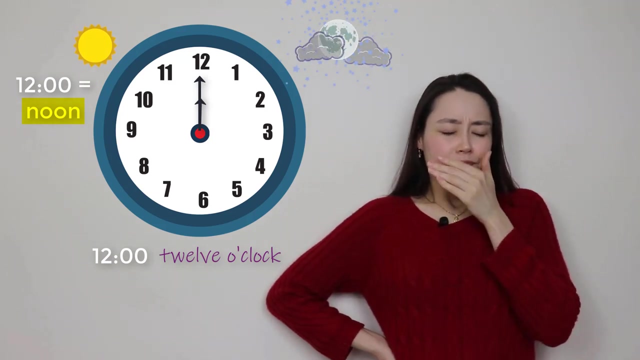 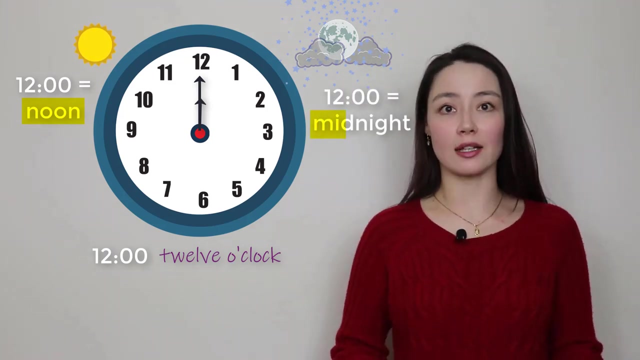 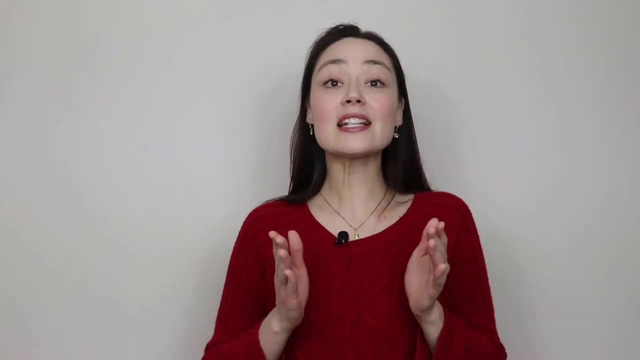 country, but in the USA and in the UK twelve o'clock is lunchtime. We can also say noon. Twelve o'clock in the afternoon is noon. I'll see you tomorrow at noon. What time is it? Twelve o'clock? It's midnight. I went to bed at midnight. Let's 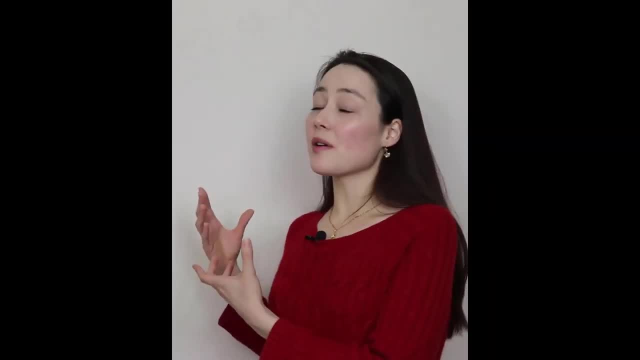 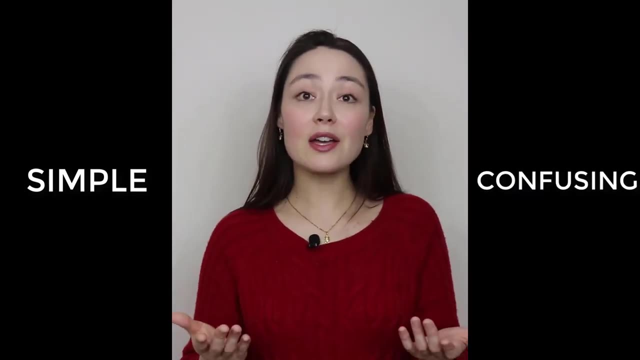 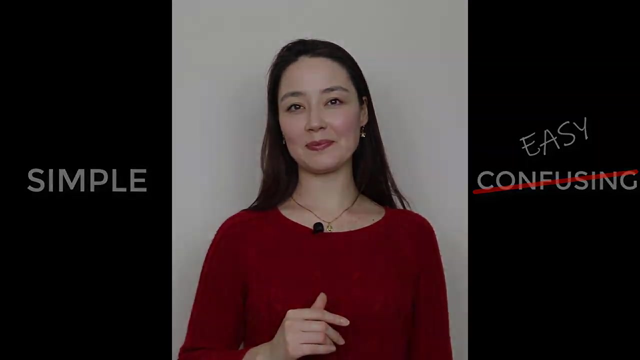 get more specific. We have a very simple way. There's also a more confusing way, But actually this is a very simple way. There's also a more confusing way, But actually this is very easy. Let's go through both step by step. I have my clock. I'm going to use a. 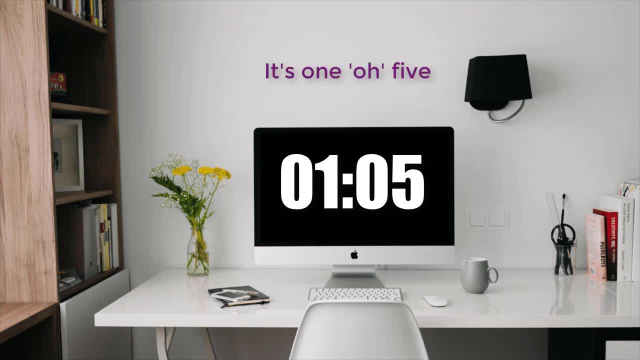 digital clock here. Now it's one o'five. We pronounce the zero o. Now it's one ten. Now it's one, fifteen, It's one, twenty, It's one forty-five. You can always read the time from left to right. With every time It's eight, twenty. 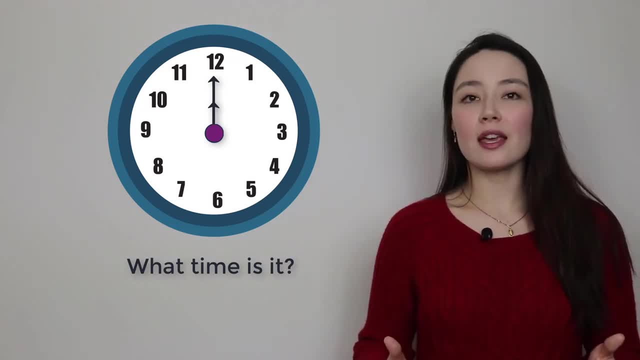 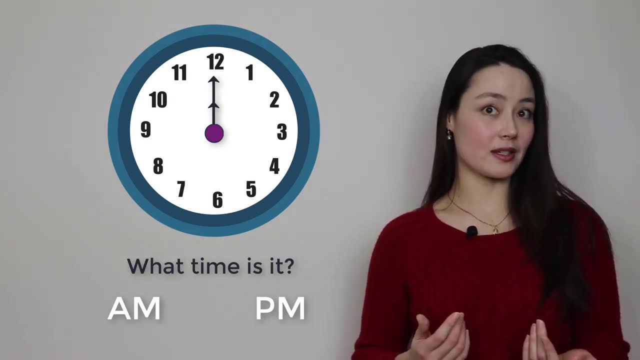 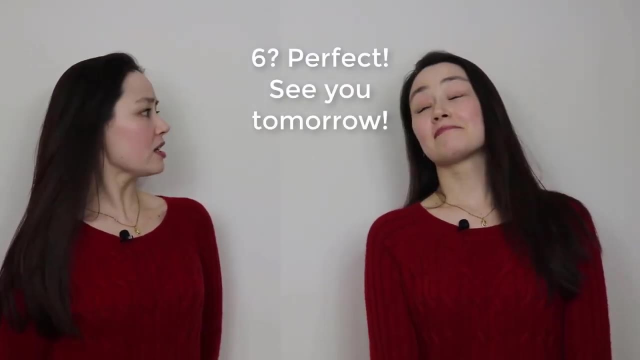 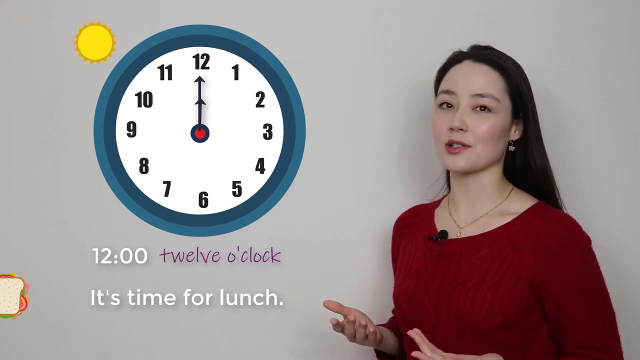 to be very specific, we can say am and pm, But normally when you're speaking it's obvious. Okay, Arnel, I need you here tomorrow at six Six, perfect, See you tomorrow. Six am am Twelve o'clock. It's time for lunch, Maybe not in your. 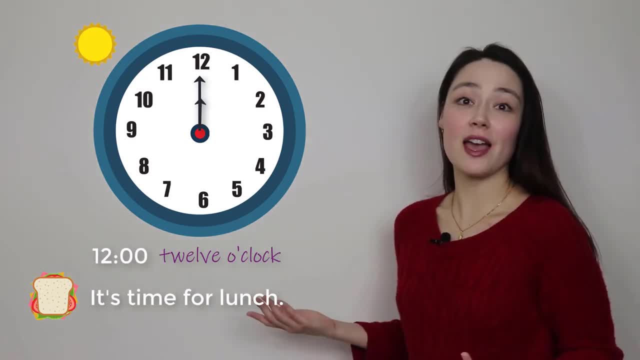 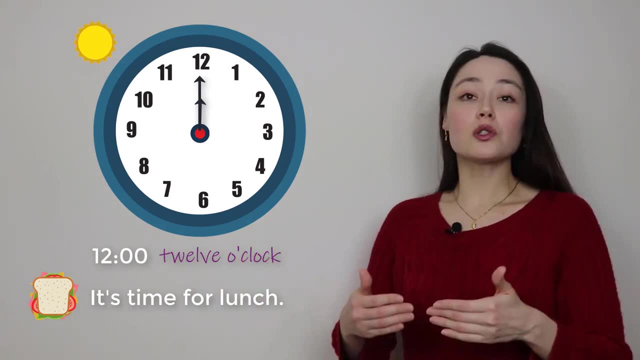 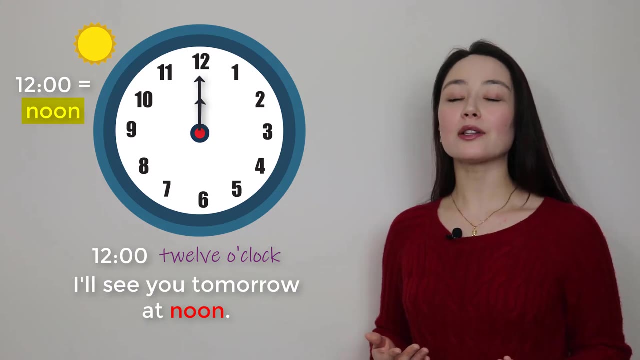 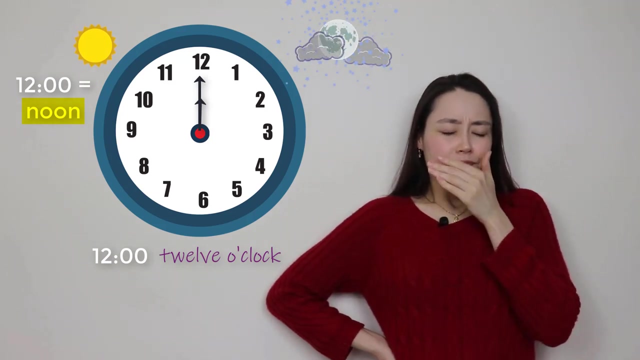 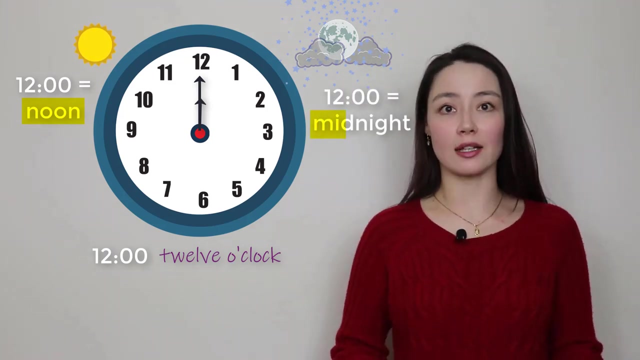 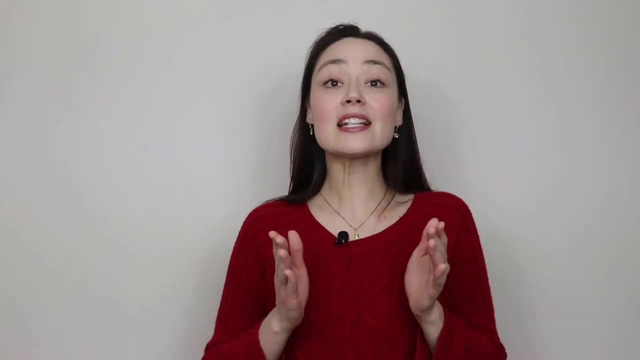 country, but in the USA and in the UK twelve o'clock is lunchtime. We can also say noon. Twelve o'clock in the afternoon is noon. I'll see you tomorrow at noon. What time is it? Twelve o'clock? It's midnight. I went to bed at midnight. Let's 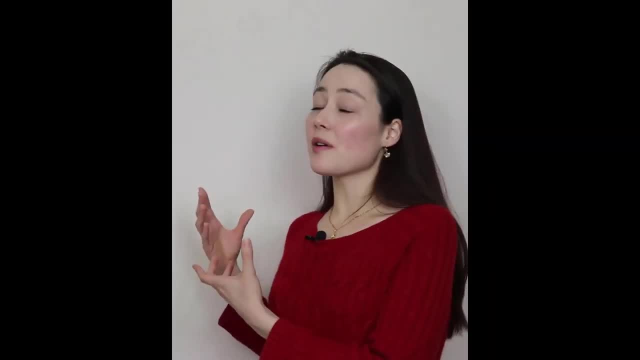 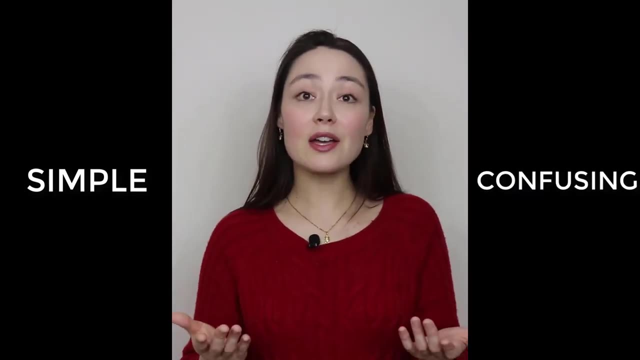 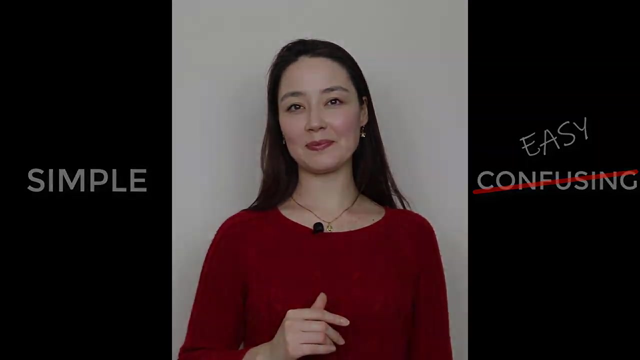 get more specific. We have a very simple way. There's also a more confusing way, but actually this is a very simple way. We have a very simple way. There's also a more confusing way, but actually this is very easy. Let's go through both step by step. I have my clock. I'm going to use a. 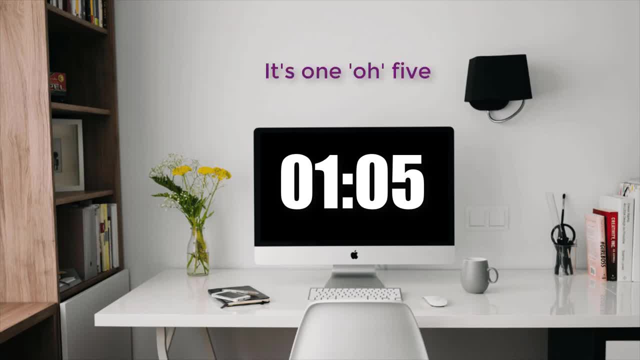 digital clock here. Now it's one o'five. We pronounce the zero o. Now it's one ten. Now it's one, fifteen, It's one, twenty, It's one forty-five. You can always read the time from left to right. With every time It's eight, twenty. 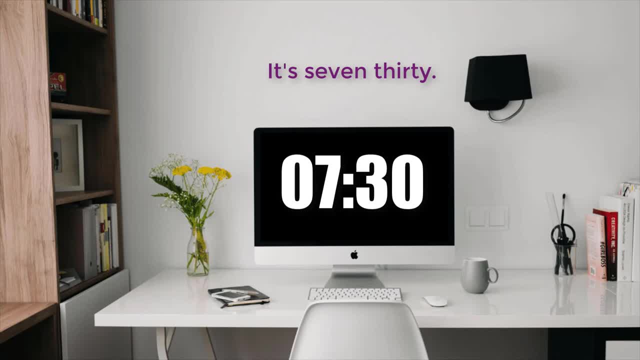 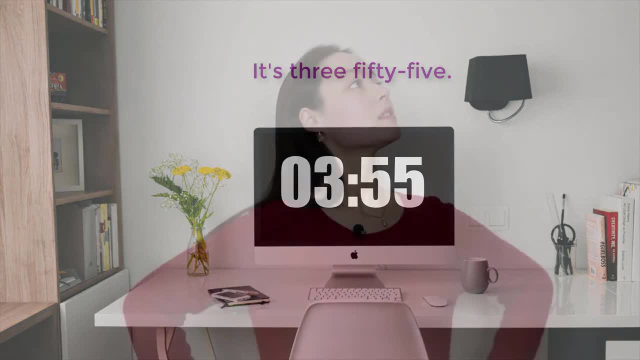 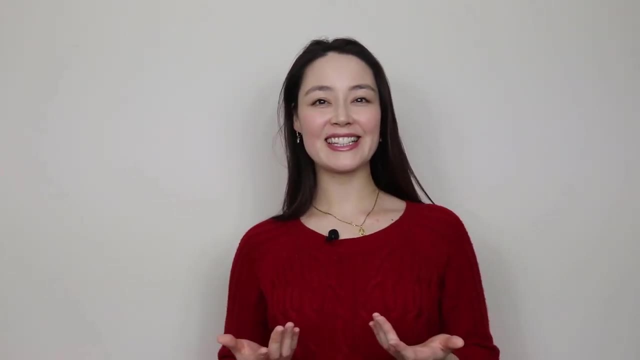 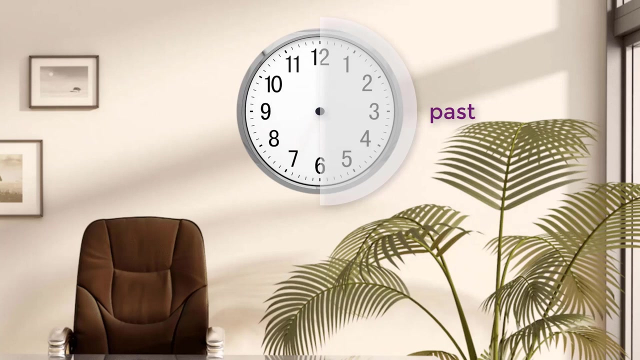 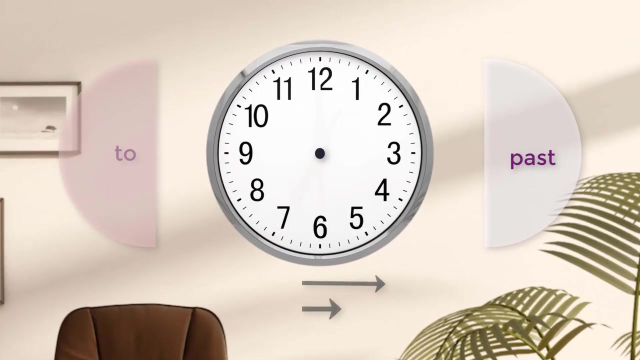 It's seven, thirty It's four, twenty-two, It's ten, ten, It's three, fifty-five. But of course there's another way. Let's take a look. I have my clock. This part is past. This part is two. Now let's have the hour hand at one. It's five past one. 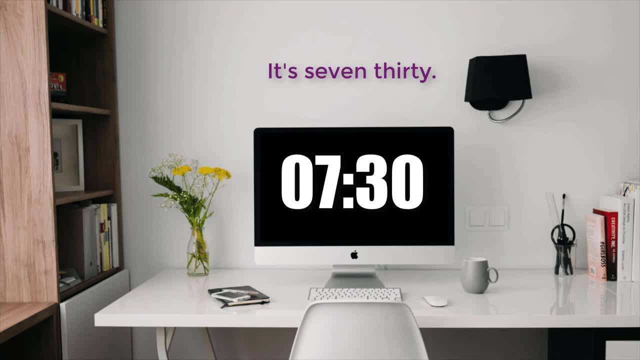 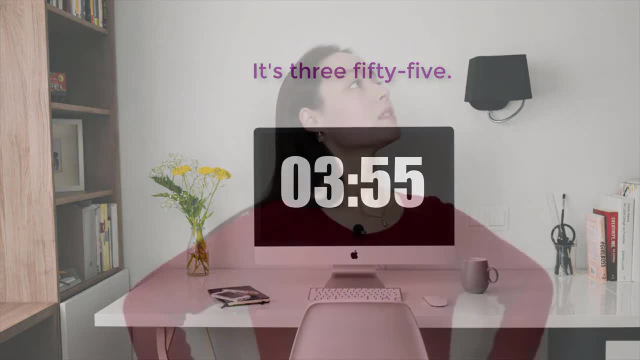 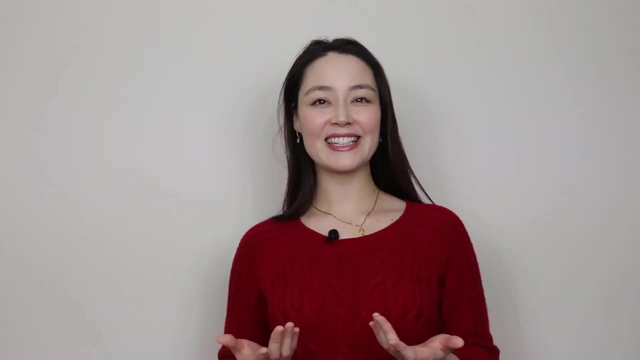 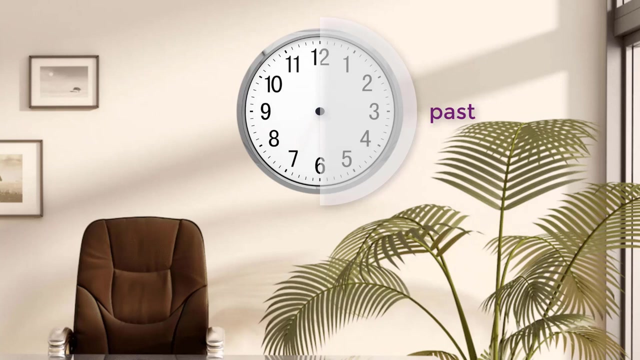 It's seven, thirty, It's four, twenty-two, It's ten, ten, It's three, fifty-five. But of course there's another way. Let's take a look. I have my clock. This part is past. This part is two. 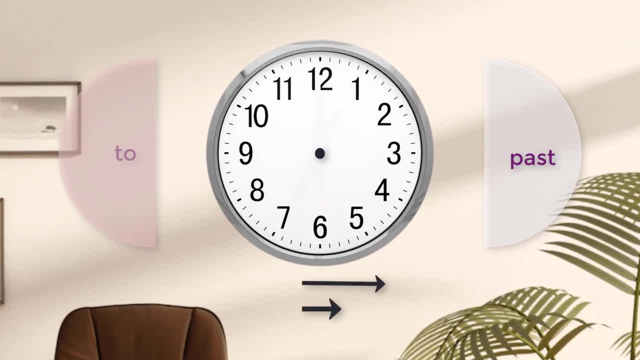 Now let's have the hour hand at one. It's five past one, Ten past one. It's quarter past one. Fifteen is always quarter past. It's twenty past one. It's twenty-five past one. It's half past one. 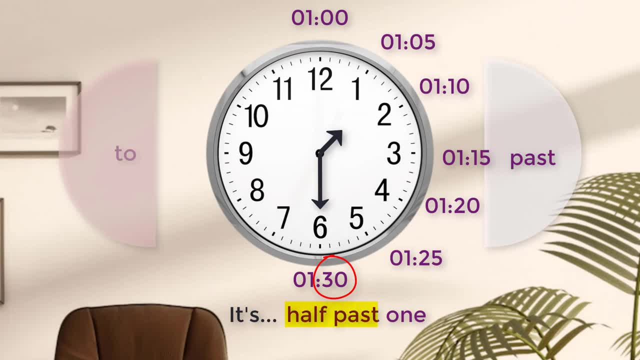 Thirty is always half past. Let's continue. It's twenty-five to two, It's twenty Two-two. It's quarter to two. Forty-five is always quarter to It's ten to two. It's five to two. Now it's two. 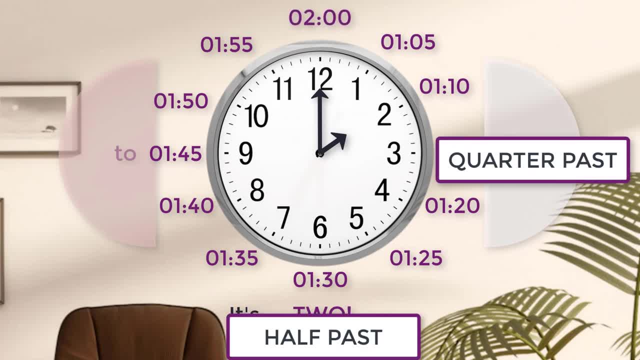 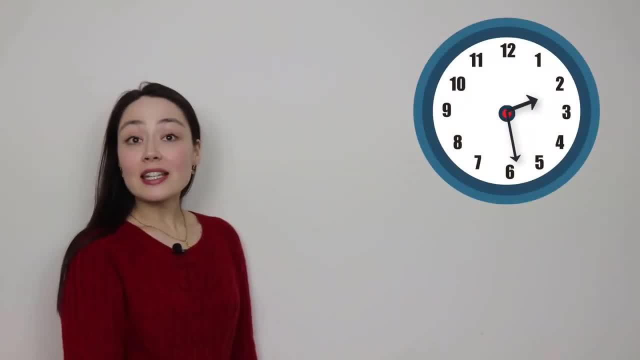 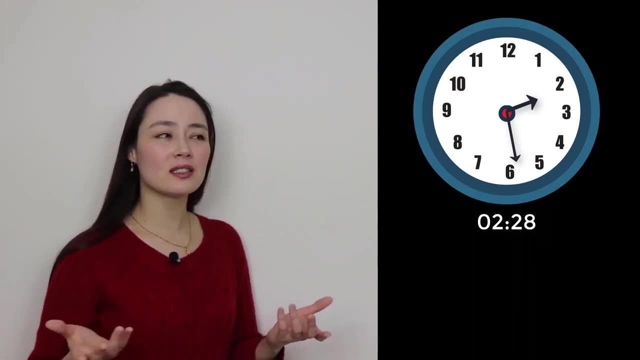 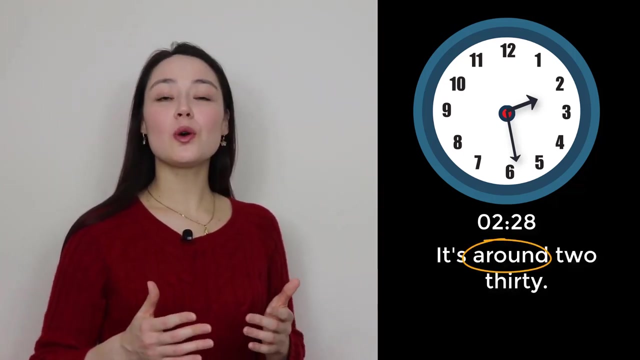 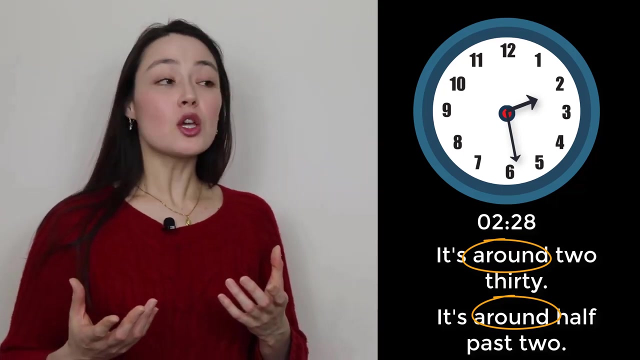 Always remember quarter past, half past, quarter to Now. it's two-twenty, Twenty-eight. Is it really necessary to be so specific? Usually, no. It's around two-thirty, It's around half past two. Whenever we're telling time, you could always use around to give a general period. 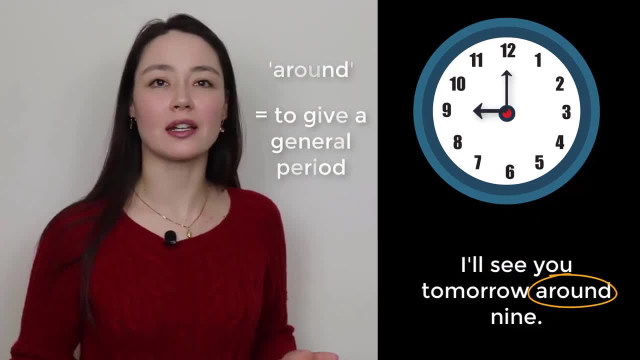 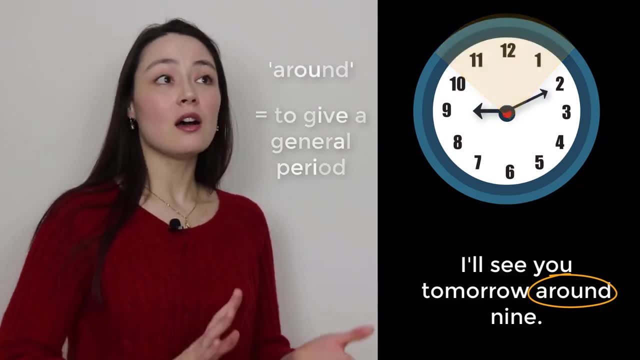 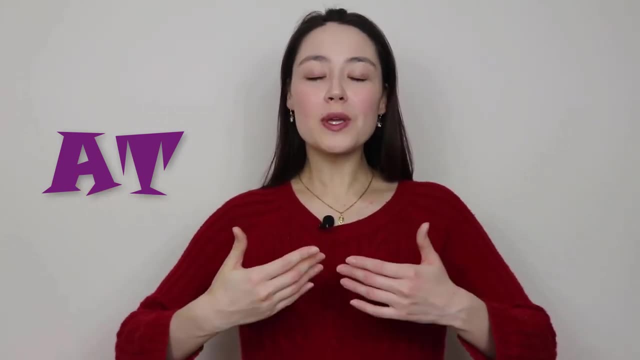 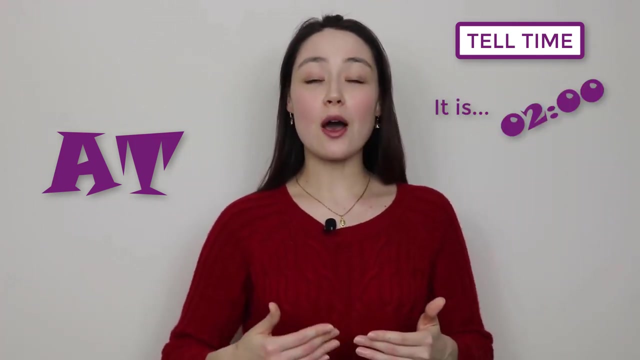 I'll see you tomorrow around nine. This could mean ten to nine, This could mean ten past nine, Around nine At. Of course, when we tell the time, we say it is Now, it is two, Now it is four. 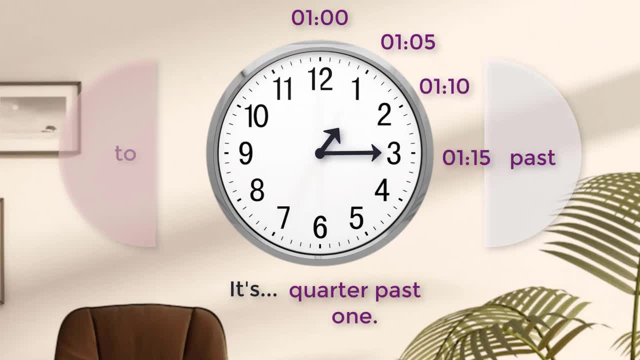 Ten past one. It's quarter past one. Fifteen is always quarter past. It's twenty past one. It's twenty-five past one. It's half past one. Thirty is always half past. Let's continue. It's twenty-five to two. It's twenty to two. It's quarter to two. 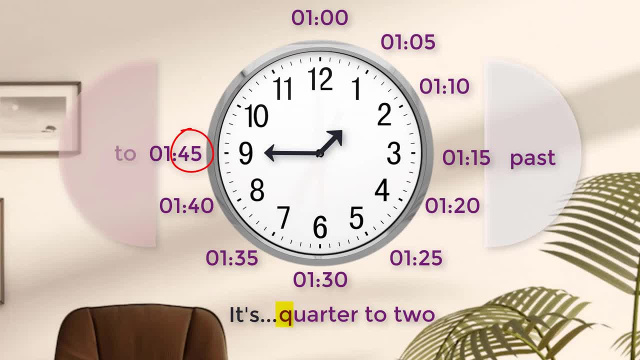 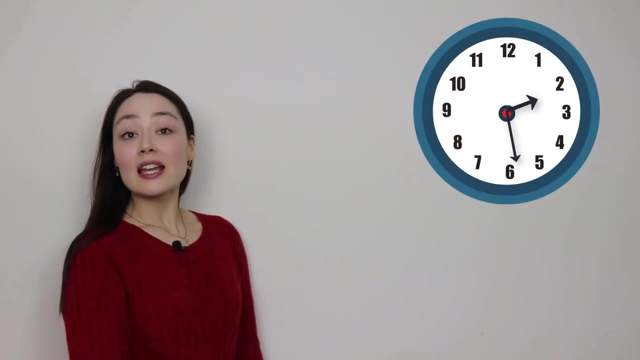 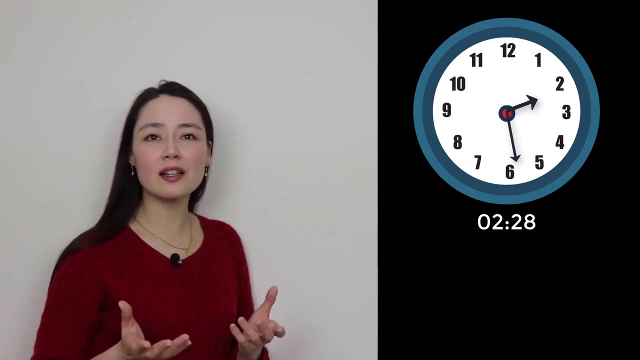 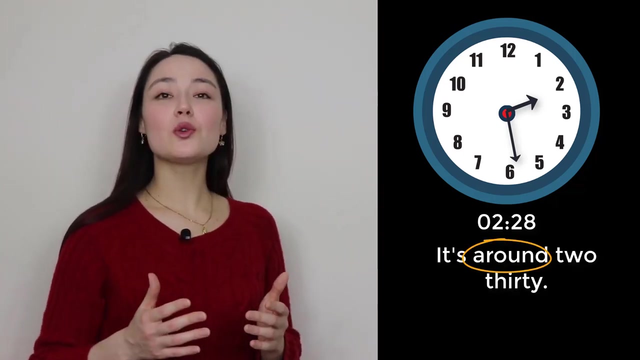 Two. Forty-five is always quarter to. It's ten to two. It's five to two. Now it's two. Always remember quarter past, Half past, quarter to Now. it's two twenty-eight. Is it really necessary to be so specific? Usually no. It's around 2.30.. It's around half past 2.. Whenever. 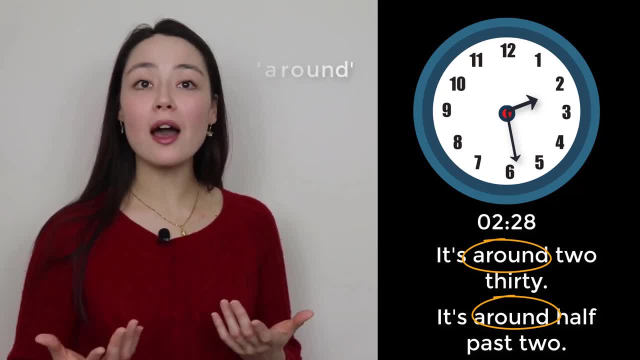 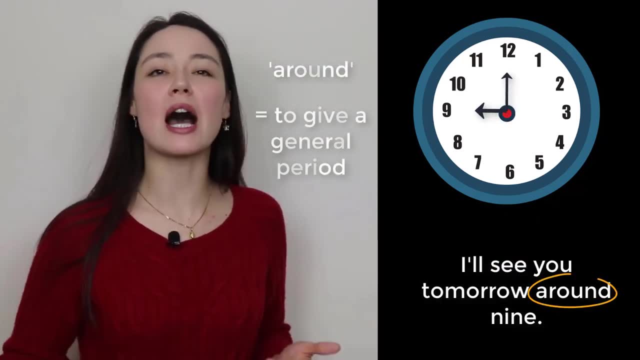 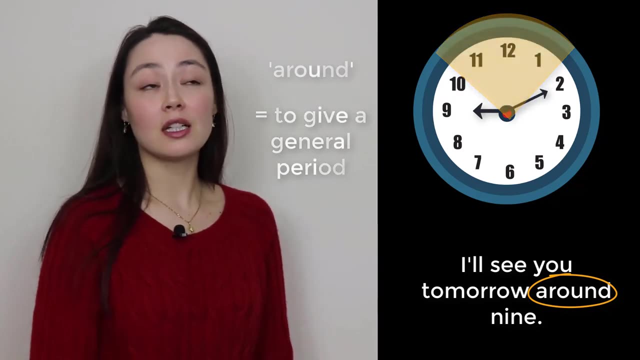 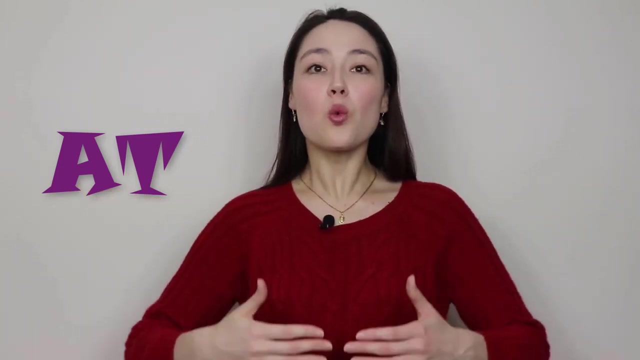 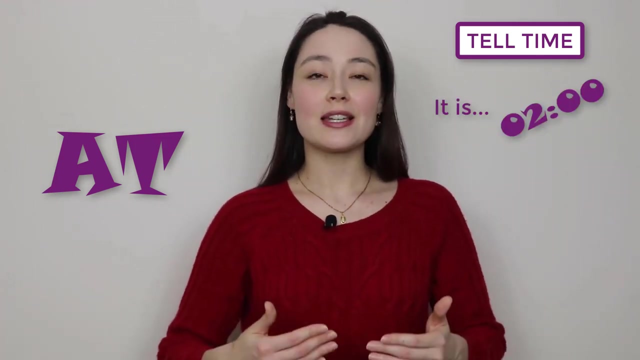 we're telling time. you could always use around to give a general period. I'll see you tomorrow around 9.. This could mean 10 to 9.. This could mean 10 past 9.. Around 9.. At, Of course, when we tell the time we say it is Now, it is 2.. Now it is 4.. But 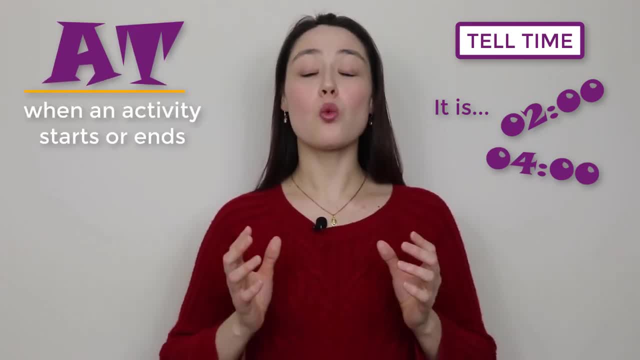 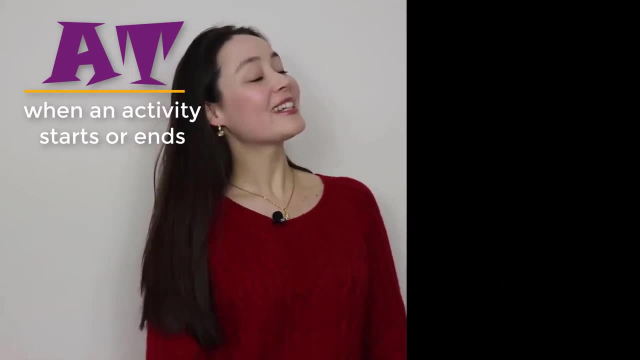 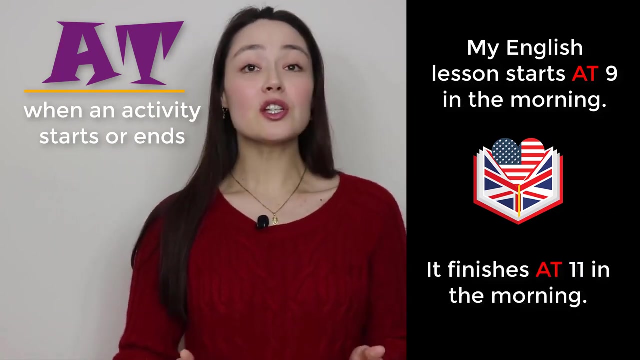 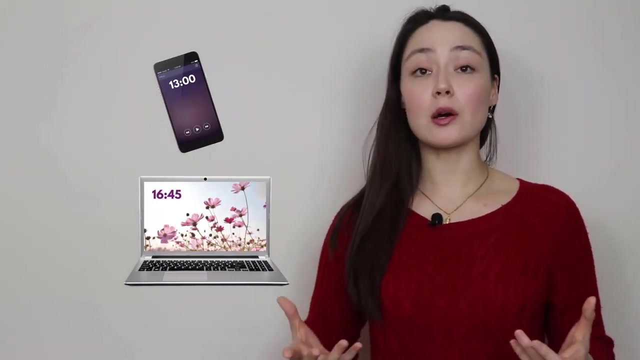 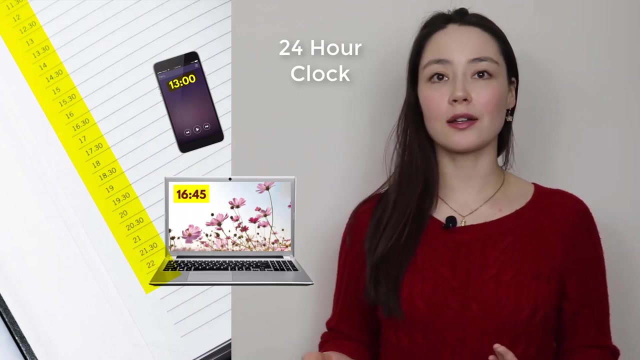 we use at when we want to say when and activity starts or ends. My English lesson starts at 9 in the morning. It finishes at 11 in the morning. Many of our phones, computers, schedules etc. use the 24-hour clock, But in English. for.